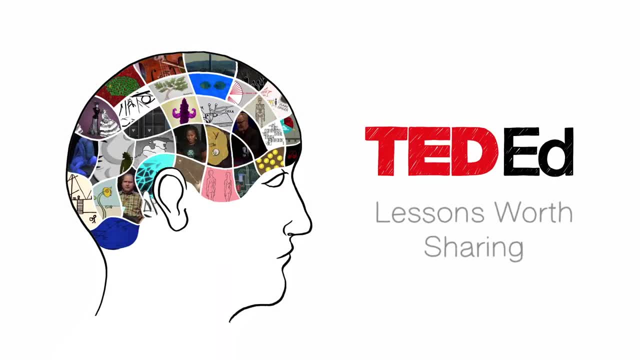 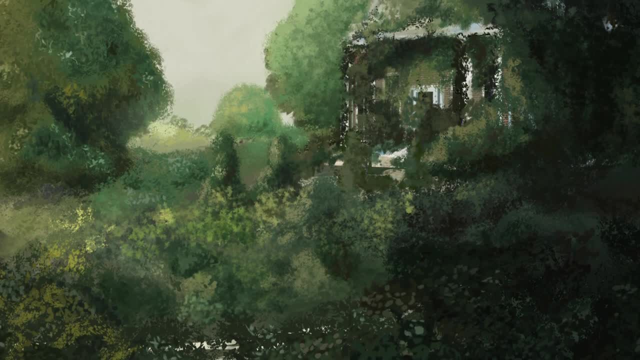 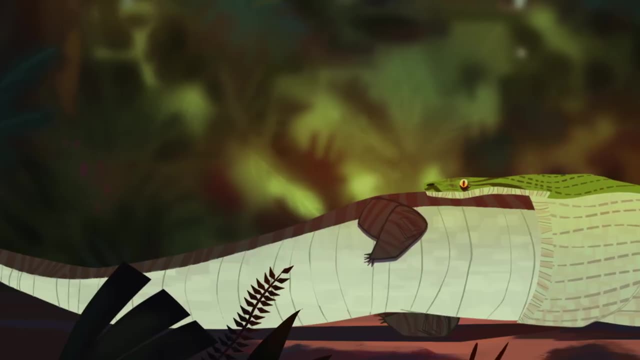 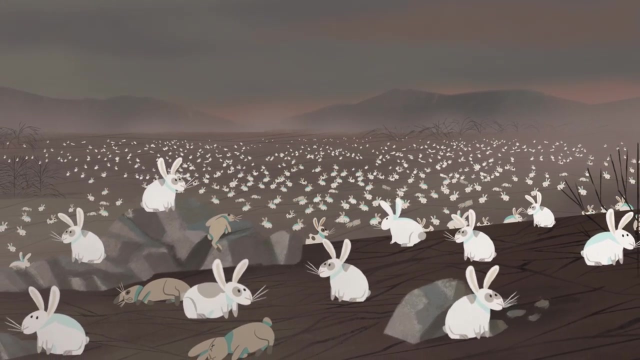 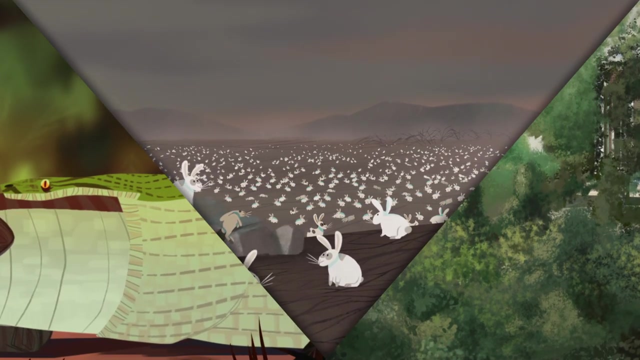 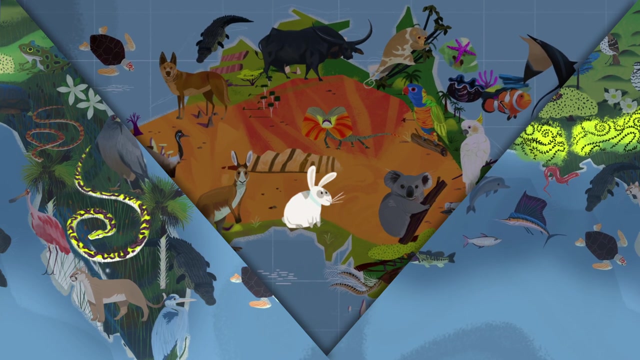 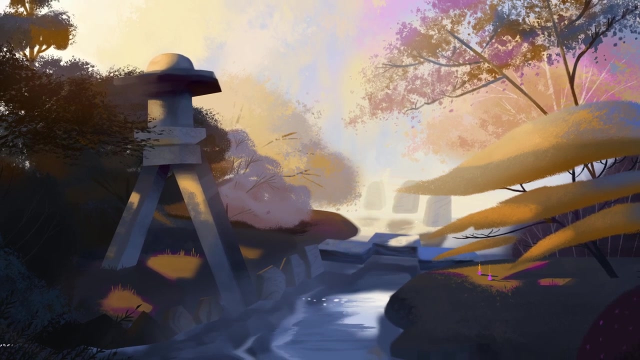 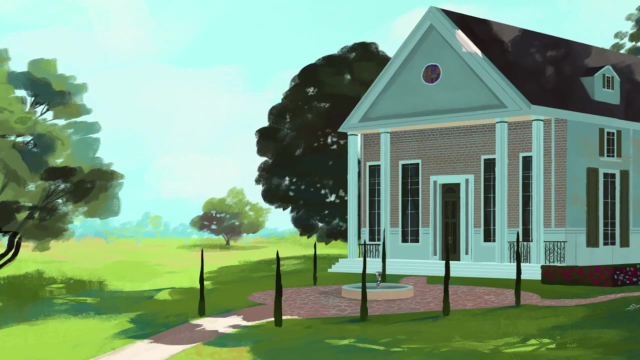 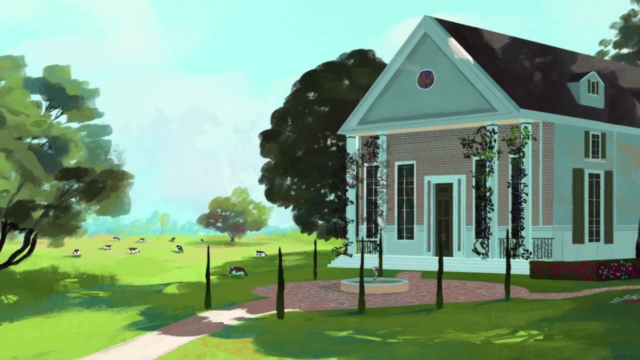 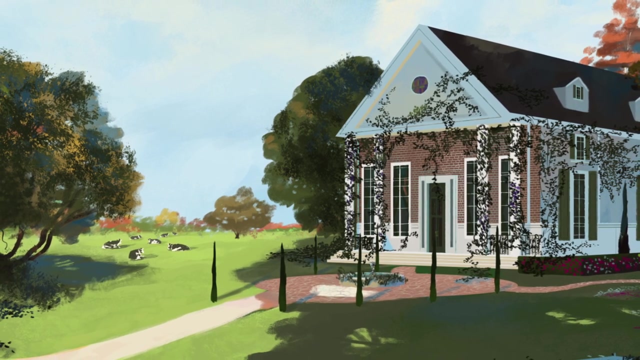 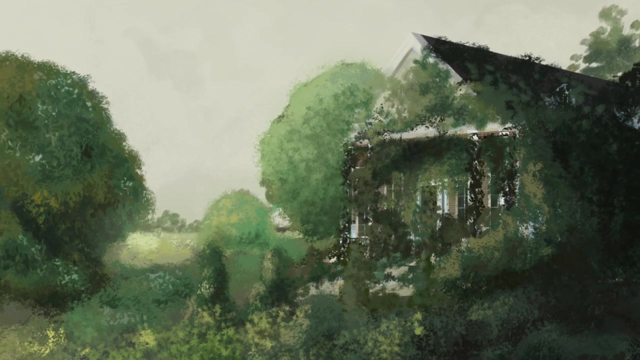 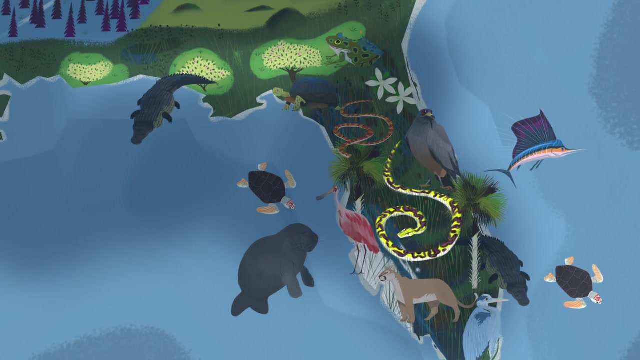 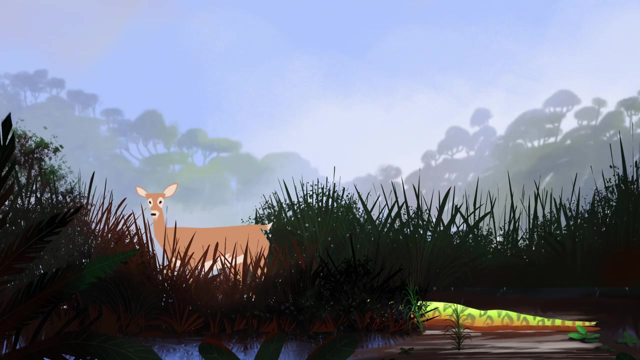 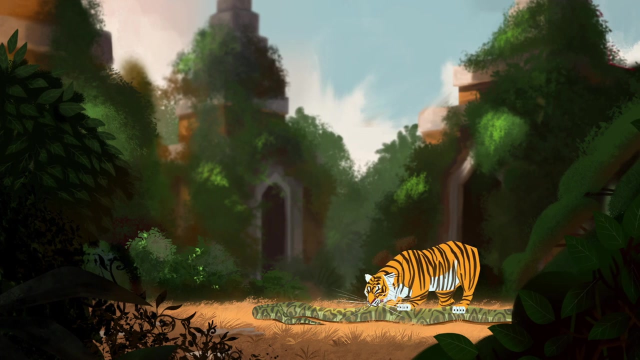 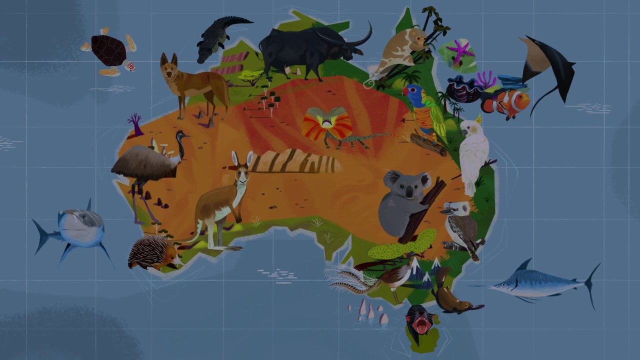 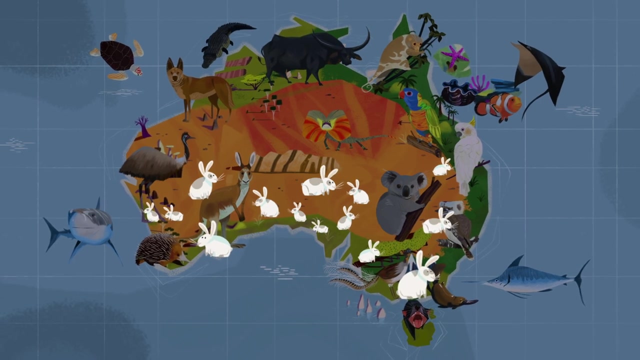 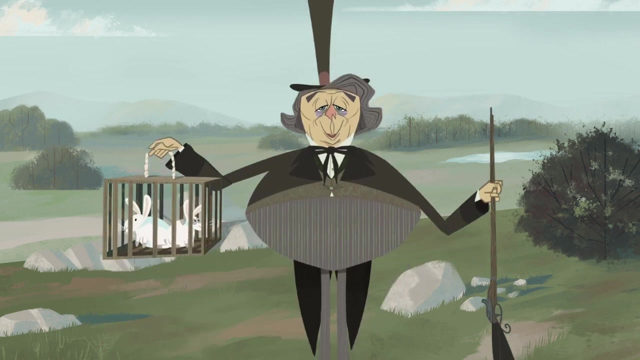 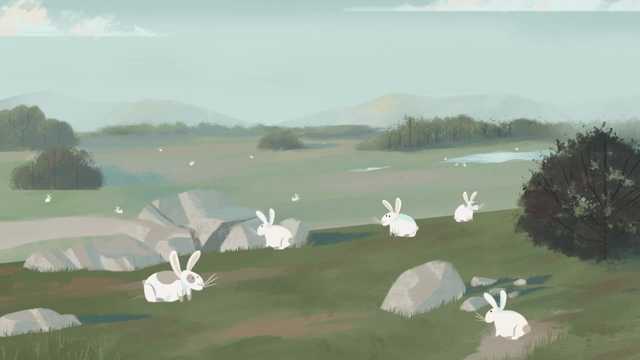 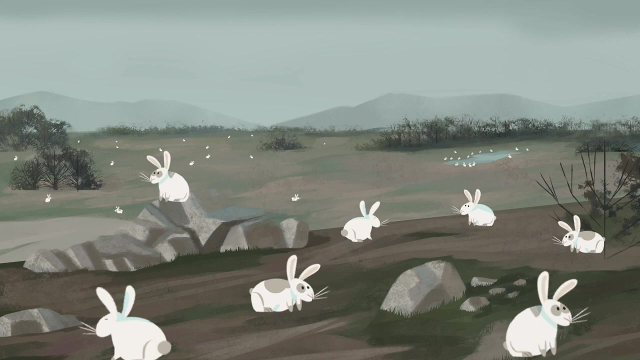 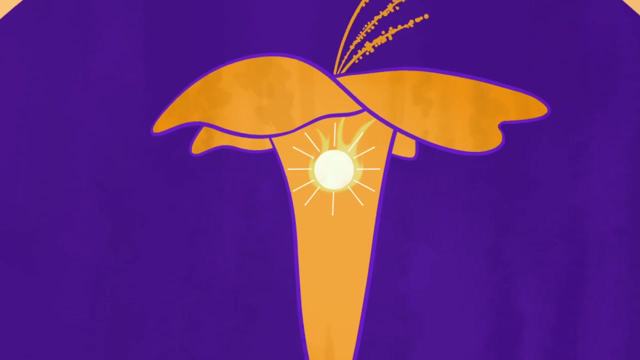 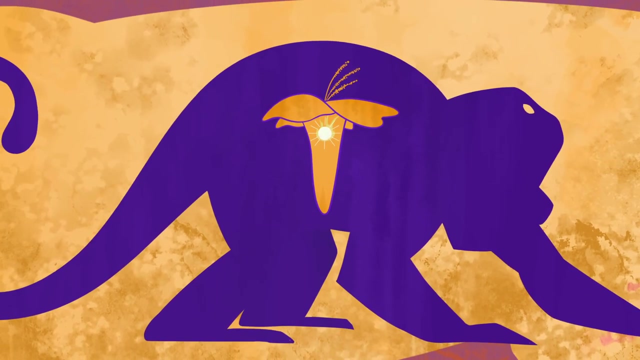 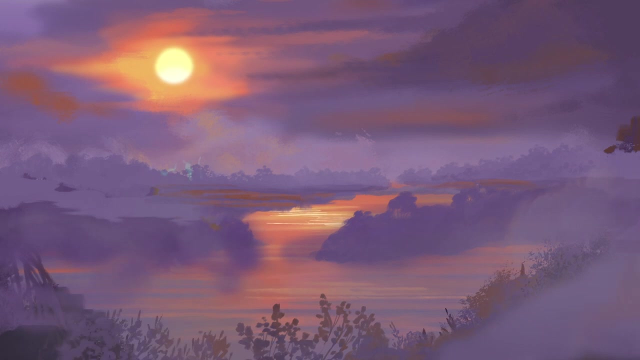 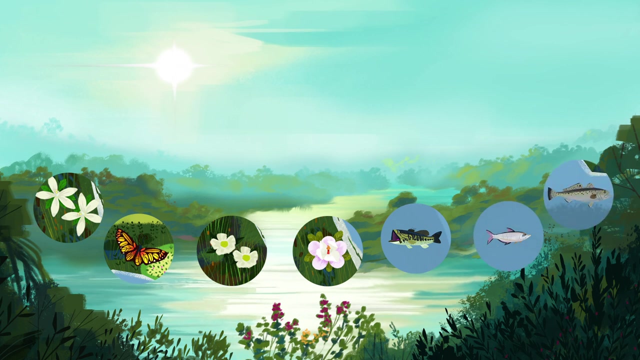 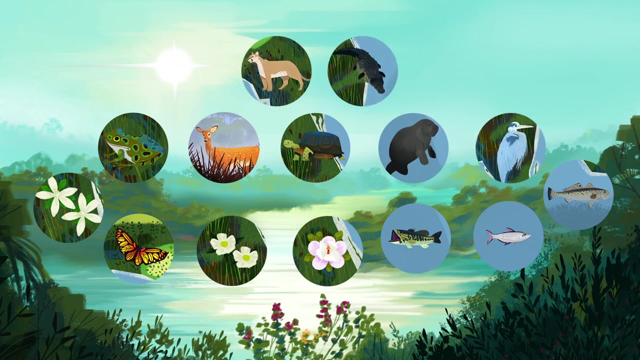 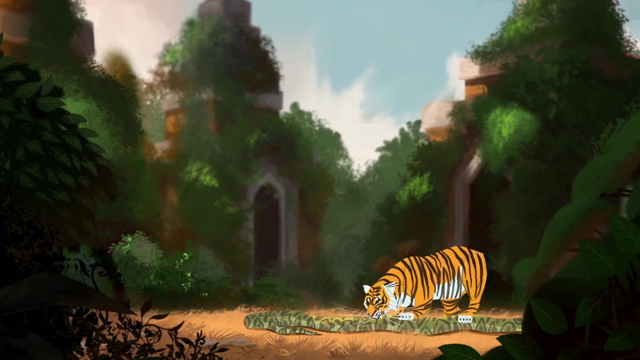 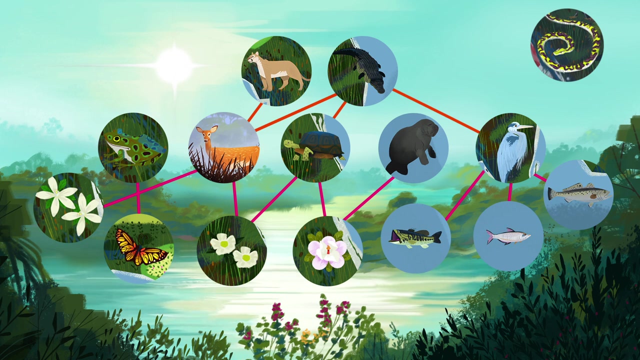 Captioning provided by Disability Access Services at Oregon State University. at Oregon State University. Captioning provided by Disability Access Services at Oregon State University. at Oregon State University. Captioning provided by Disability Access Services at Oregon State University at Oregon State University. Captioning provided by Disability Access Services at Oregon State University.